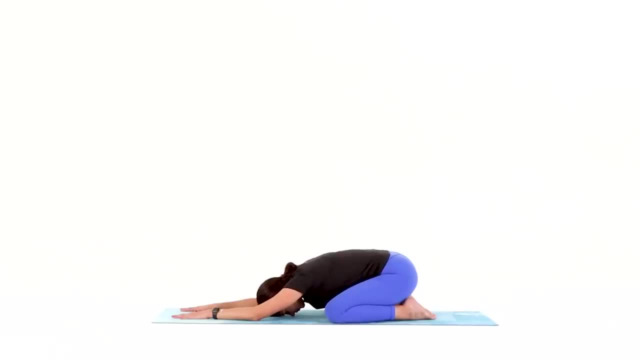 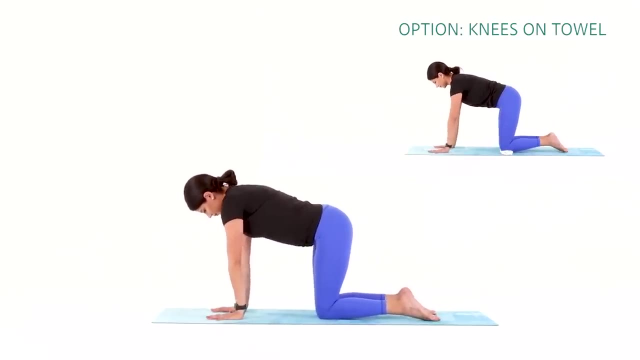 your nose And relax. And out through your mouth, Relax, And out through your mouth: Relax. Now lift up your head to the back. Watch your body relax. Do not lift the knees up more. As you cool down your belly muscles, raise your arms and make sure your hands are parallel with. 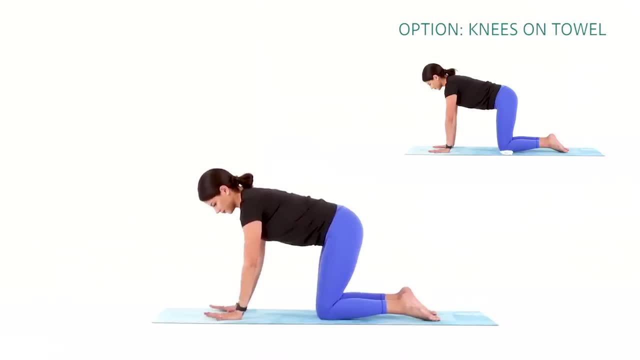 one another. Now, as you exhale, sit down. Your hands are directly underneath your hips, so your thighs are parallel with each other. Your hands directly underneath your shoulders, So your arms are parallel with one another. js, every time you use yogi hands on your mat. now look at your elbows. make sure you're not resting. 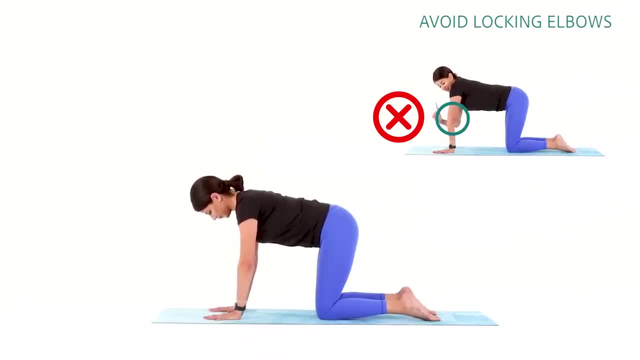 in locked elbows there's just a tiny little bend, just enough so that all the muscles around your elbows are engaged and they will strengthen and support your elbow joint over time. then, with these strong arms, strong hands, pull your navel in towards your spine. this will help. 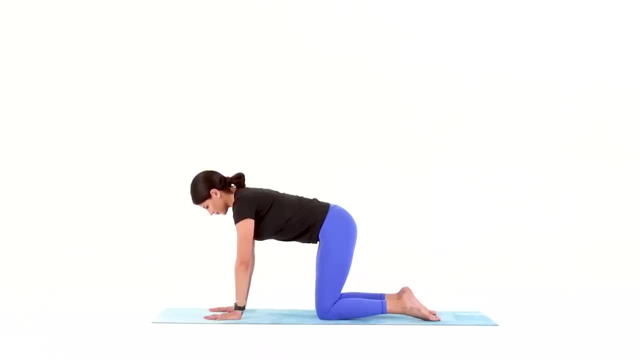 to lift your belly up and hold your core into place so you're not letting your belly droop down towards the mat. your core is engaged. then keep that engagement and extend your right leg straight behind you, driving back through your right heel so your leg is in line with your spine, and hold 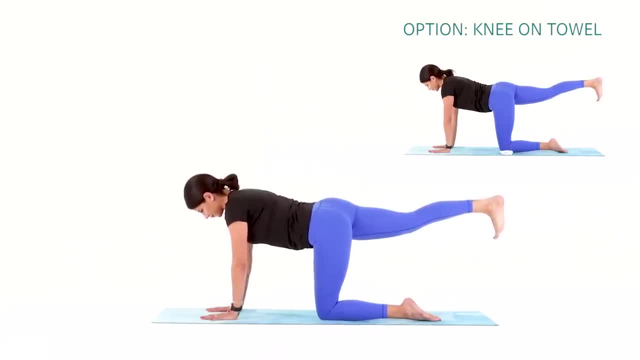 keep your belly. pulling in neck is in line with your spine. yogi hands are strong on your mat. three, two, three, four, one. then lower your right knee back down into your tabletop and switch sides. extend your left leg straight back behind you. drive back through your heel. 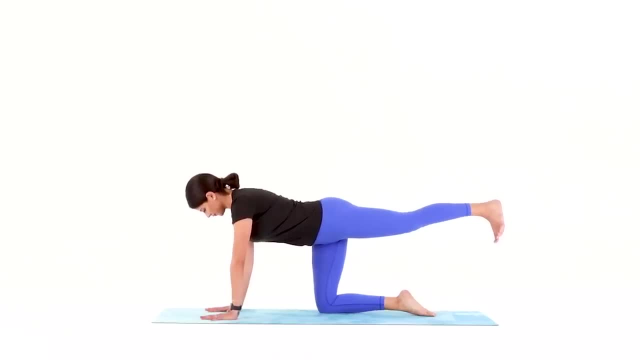 left leg in line with your spine and all the rest of your tabletop is still strong and engaged, with your belly pulling in and your breath calm. three, two, one. come back to tabletop. well done from here. five, six, seven, six. very good, now how to lift your back up. 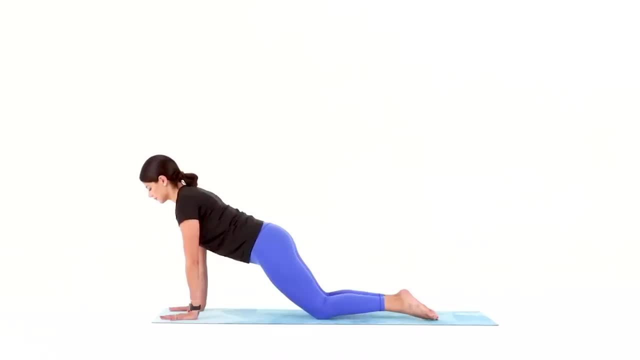 put your head back into your seat and watch this video with me. I want you to keep the plank in your body as much as you can and just bend your elbows directly back as you lower down halfway, until your elbows touch your ribs, and then stop there and hold. 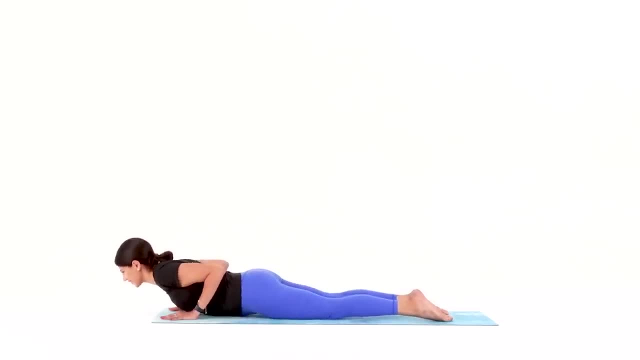 This is modified- low plank and then lower all the way down to your belly. Well done, Now press back into your hands to lift up into your tabletop and then take a seat on your heels or just stand on your knees and just shake your hands out That high to low plank, just bending your elbows back. 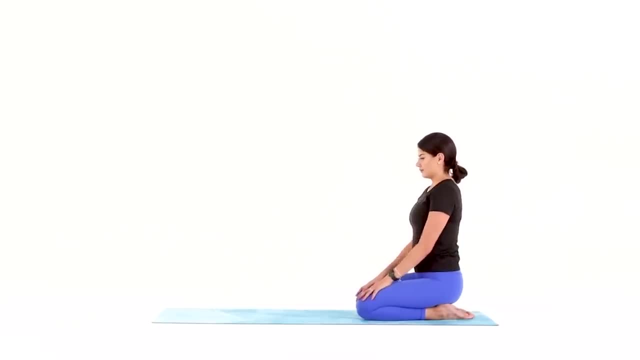 and lowering your plank halfway down is a common sequence of yoga poses that you'll see in a power yoga class, So it's important that you learn how to do them properly, and we're modifying so that we can build a foundation of strength. So if you watched the first time through, come and join me. 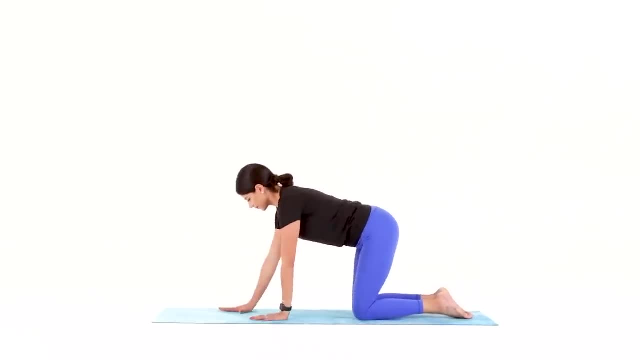 for the second time. If you've done it the first time through, come and join me for the second. Let's come forward into a high plank, together Modified, with our knees down. find that flat back as if there's a plank of wood touching the back of your knees, your hips, behind your shoulders. 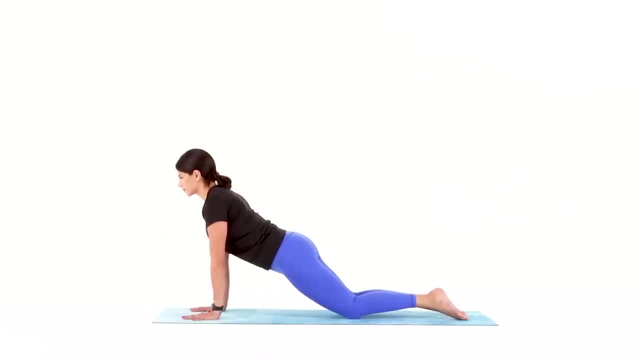 and the back of your head. Maintain that plank and bend your elbows directly back as you lower your body halfway down towards the ground. Pause when your elbows touch your ribs. then lower all the way down to your belly. That's a lot of work, but you did it From here. set up for a low cobra. 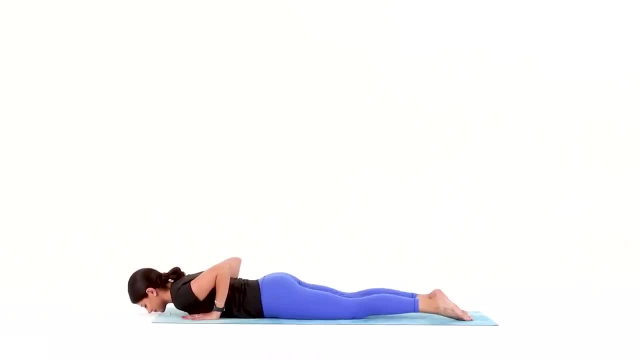 Keep your hands underneath your shoulders and zip your legs and feet together to touch behind you and press the tops of your feet down into the mat so much that your knees lift up slightly. Keep pushing down through the tops of your feet and keep your legs engaged this way. 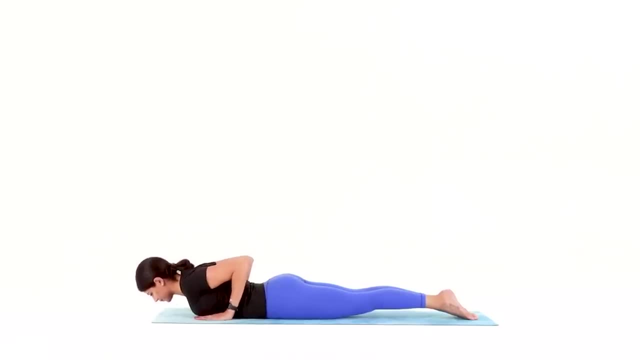 And then pinch your elbows together behind you, as if you were trying to get them to touch and feel your shoulders open up. Now use your back strength to lift your chest and shoulders up off the mat and keep your gaze just a few inches out in front of your mat so you don't crane your 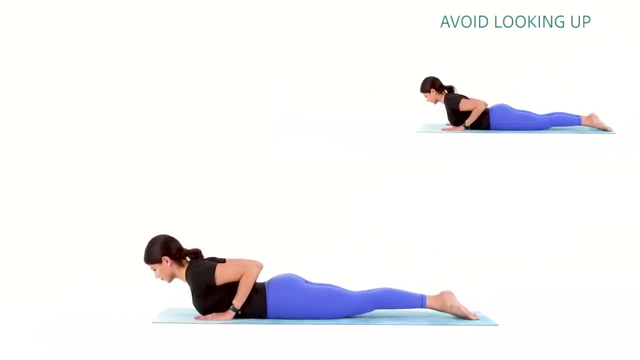 neck. The strength of your back is keeping you lifting in this pose, even with your hands down on your mat, And feel yourself gently, bob, as you breathe. This is called low cobra. For three: you should feel the strength in your back. Two, but not strain If you're feeling. 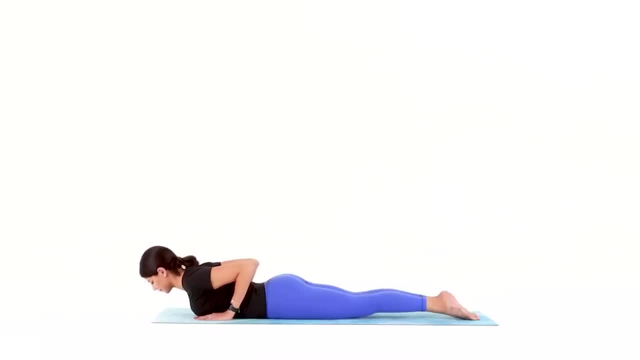 strained. you need to lower down a little more. One release and lower your right ear down to your mat. Take your arms long down by your sides and let your feet fall open for a belly shavasana, A pose of complete and total relaxation. 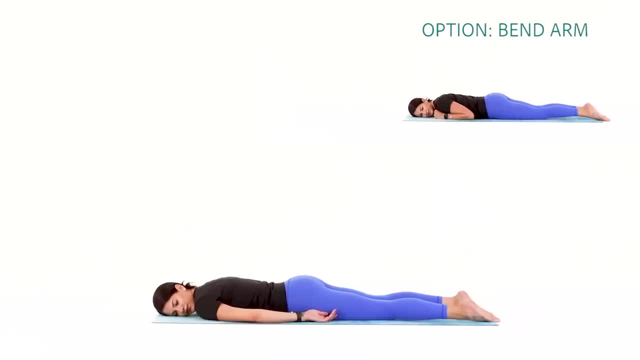 But if this feels like too big of a stretch on your neck right now, then bend your left arm and bend your right arm, And if this feels like too big of a stretch on your neck right now, then bend your left arm to place your left fist underneath your left shoulder And that. 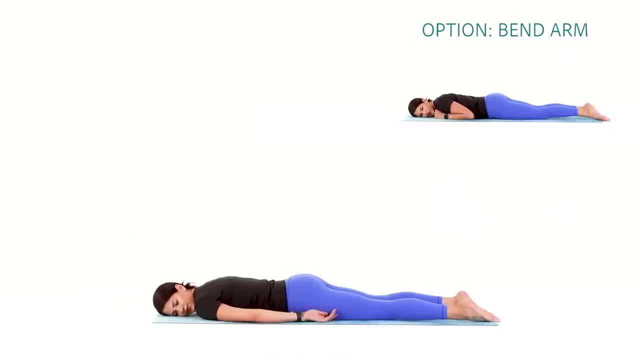 will help to reduce the intensity of the twist here. Completely relax, if only for a moment, And then draw your chin back to center, plant your hands underneath your shoulders and let's set up for a second low cobra. So zip your legs and feet together, press. 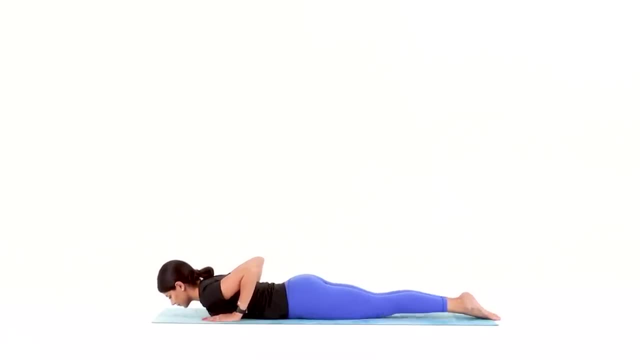 the tops of your feet down. keep your legs engaged this way and peel your chest up off the mat With your hands touching the mat, but you're not pressing into your hands. Neck is in line with your spine, so you're not crunching your neck to look forward Instead. 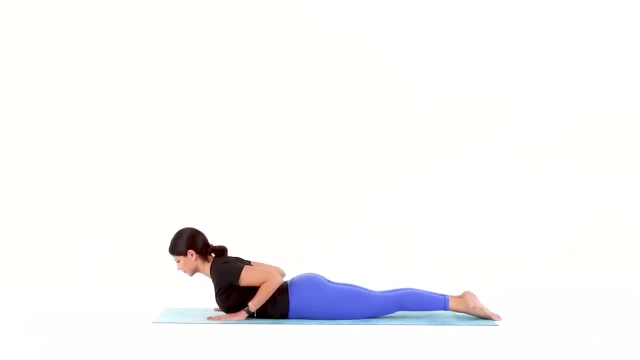 just look a few inches out in front of you. Feel yourself bob with your breath. Three: see if you can lift a little bit higher. Two: one release and lower your right ear down, Your left ear down to the mat for another belly shavasana Arms long down by your sides. 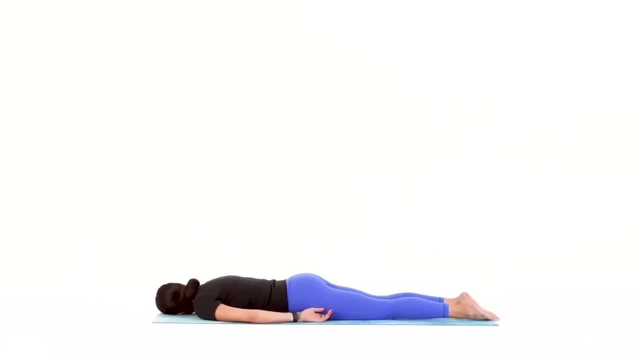 feet fall open, Total relaxation. Then draw your chin back to center, plant your hands underneath your shoulders, press into your hands to lift up into a tabletop and then set up extended child's pose with your knees wide, Big toes together behind you. 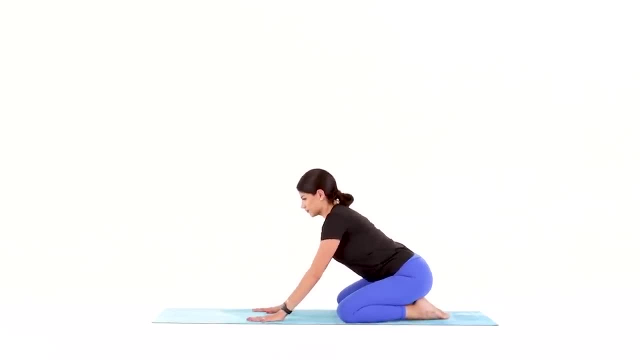 Sit your hips back, walk your hands forward, rest your forehead down onto your mat or on stacked fists and feel your breath as it creates space in your lower back. The secret to strength is the ability to hold yourself up when gravity is pulling you down. 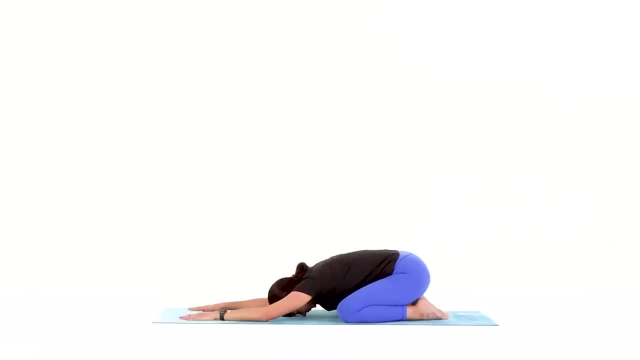 And it doesn't matter if you modified or made it easier or you took a break. You showed up and you held yourself up, even as gravity pulled you down. So I hope you enjoyed this video. If you did, please give it a thumbs up, and if you want to see more videos like this, 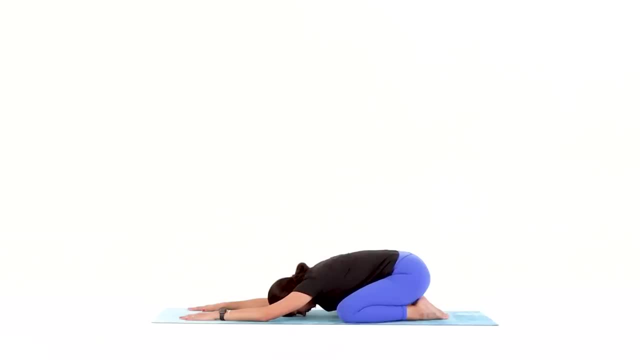 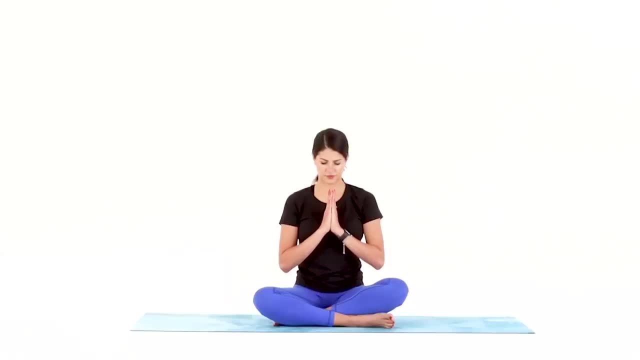 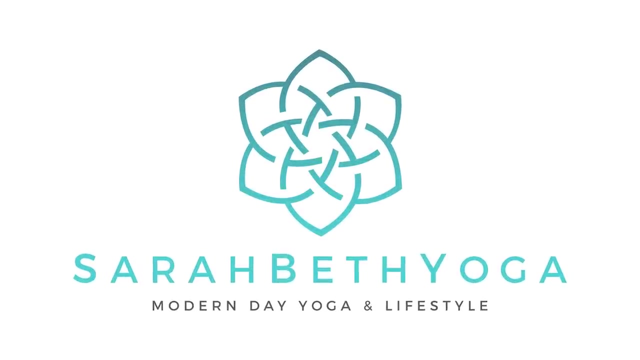 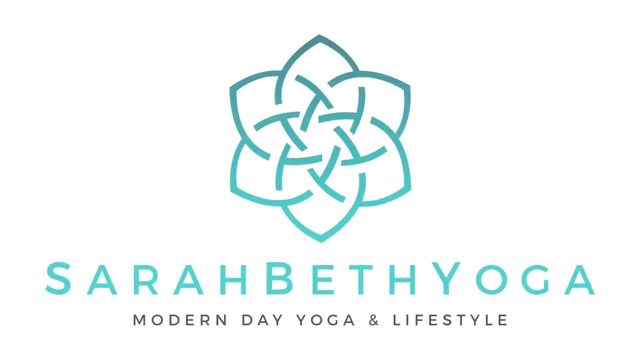 Stay safe, Stay safe, Stay safe When you are in this place in you and I am in this place in me. we are one Namaste. Well done, Hi. I'm Sarah Beth, and I'm here to help you get fit. 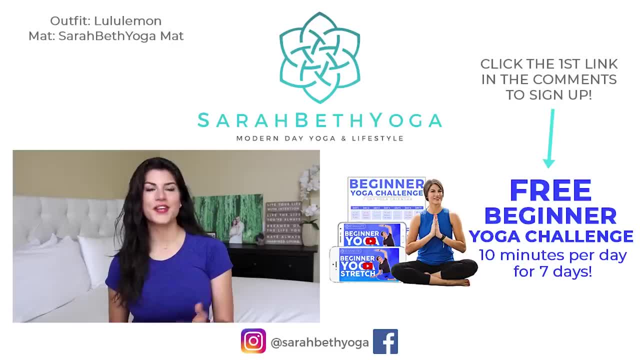 happy and healthy through yoga. I created this beginner level yoga video as an easy and fast way to wake up your body and increase your flexibility and strength. If you enjoyed this video, you're gonna love my free seven day beginner yoga challenge with simple beginner level yoga videos. 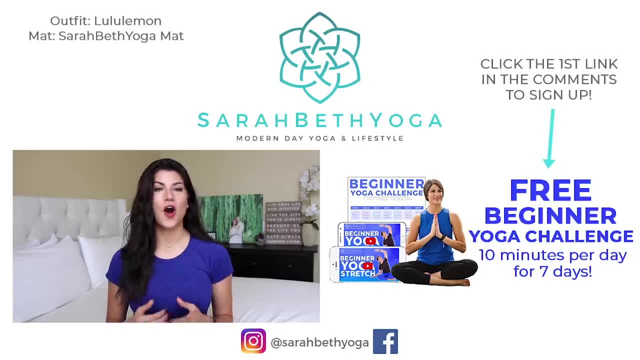 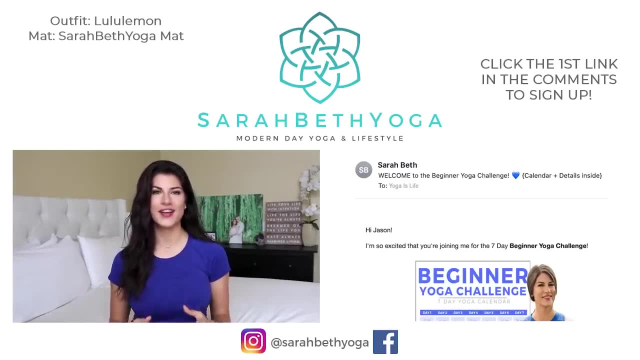 to help you get fit and flexible fast. All you need to do to get access to this challenge is click the first link in the comments below, enter your name and email and I'll instantly send you the challenge calendar and all the details. Now, did you enjoy this video? 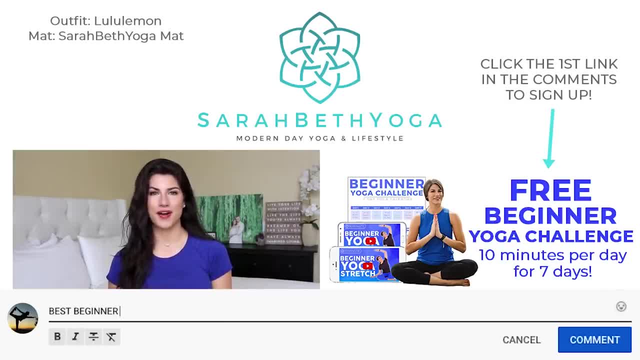 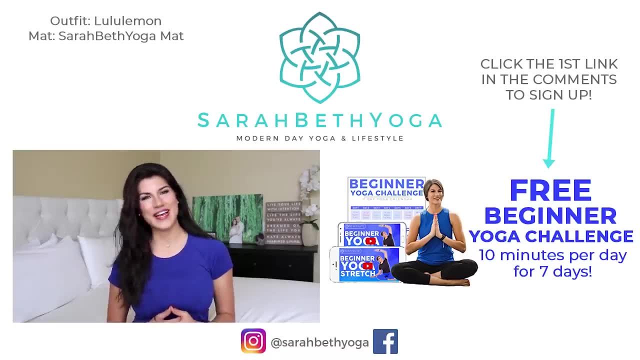 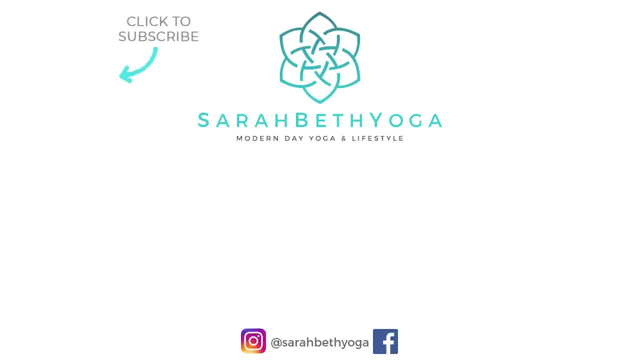 Let me know by clicking the like button below and comment with your favorite part, And don't forget to subscribe and hit that notification bell so you never miss when I upload a new free yoga video. Have a good day, Bye.